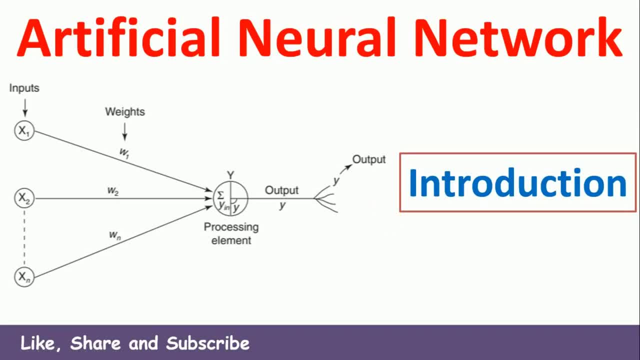 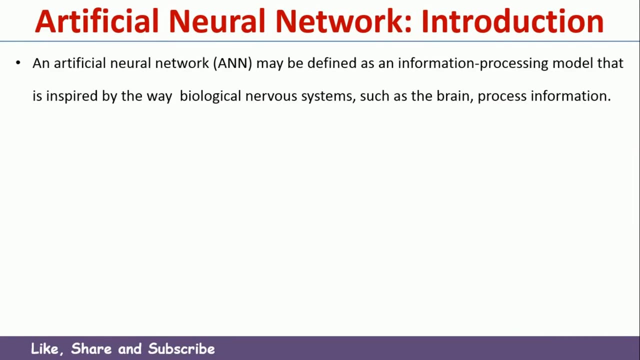 Hi, welcome back. In this video I will discuss the introduction part of artificial neural network. In the coming videos I will discuss the different concepts of artificial neural network in detail. Artificial neural network is an information processing model similar to the human brain. 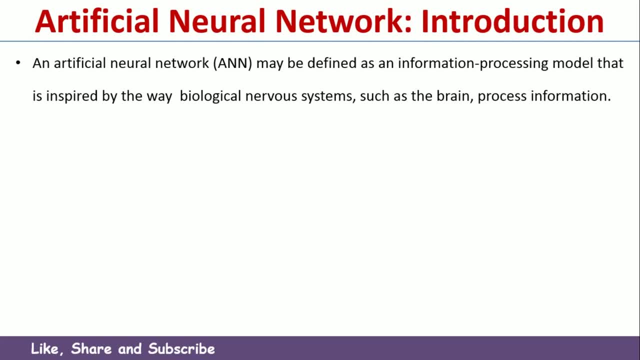 That is the way the human brain processes the information. Similarly, the artificial neural network processes the information. But the artificial neural network cannot do all the functionalities of brain, because brain is a very complex nervous system. It does a lot of computation and those computations cannot be replicated in an artificial neural network. 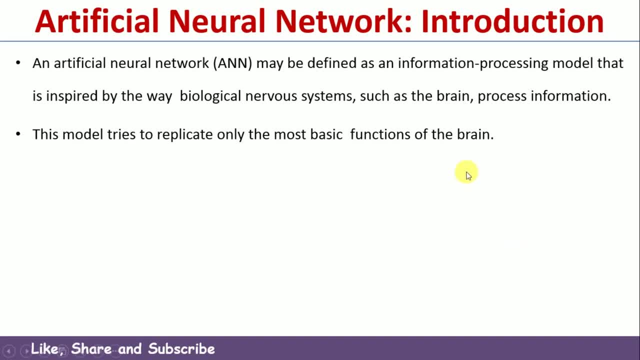 But still we can do most of the functions what brain does in artificial neural network. An artificial neural network is composed of a large number of highly interconnected processing units. Those processing units are called as neurons. Those neurons are connected so that we can solve a particular problem. 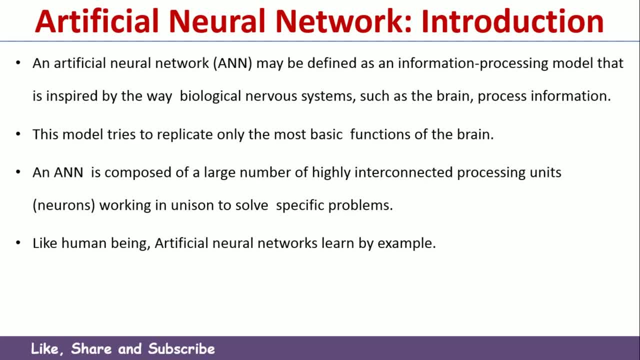 Like a human being. for example, the human being learn a particular concept or anything by experience. For example, initially, with some examples, he may learn or he may get some knowledge. But as and when he has been shown within more number of examples, the human being will learn or get more knowledge. Similar to that. 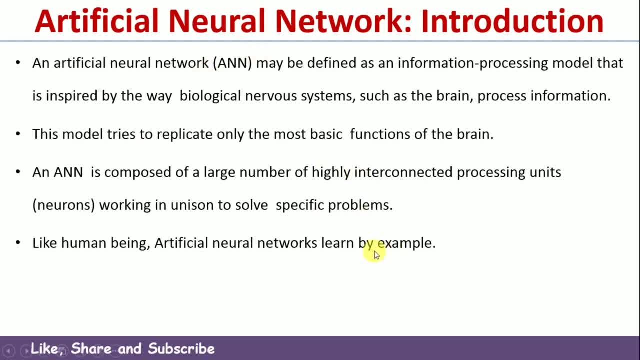 one. as and when you go on giving more and more number of example to artificial neural network, it will go on getting more and more knowledge, in this case, or it will learn more and more. An artificial neural network is configured for a specific application or to solve a particular. 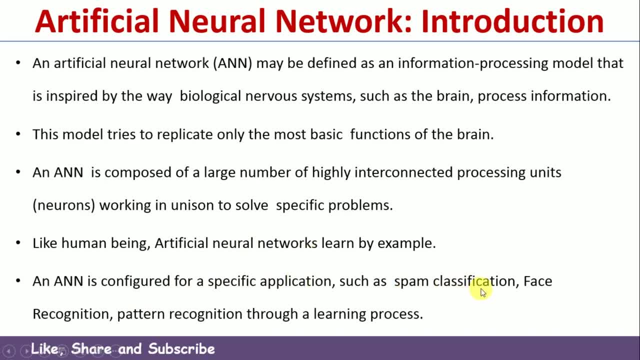 problem, That is, to solve a spam, classification, face recognition, pattern recognition or similar to such kind of any application. That is, you cannot solve all the problems using one artificial neural network. A particular artificial neural network can solve one problem at a time. That is the one. 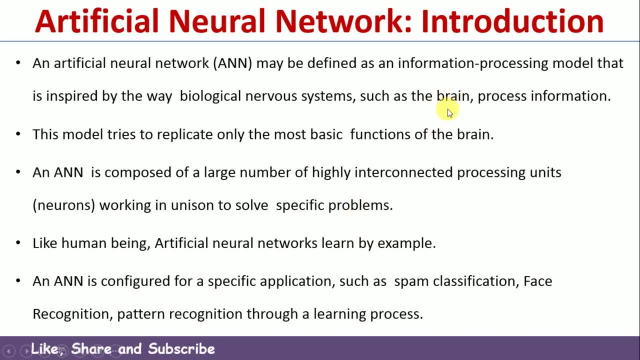 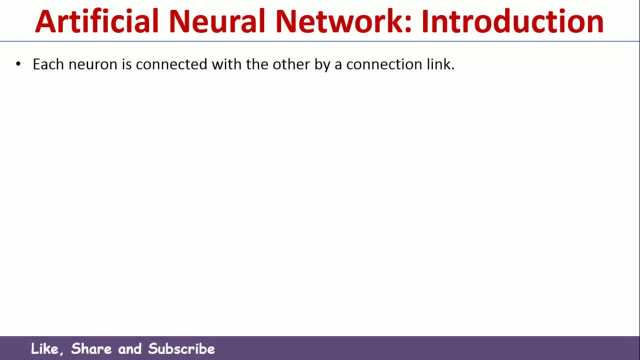 more very important part we need to remember. But brain works in such a way that it will try to solve, or it will solve, every problem over here. Each neuron is connected with other neuron with a connection link In artificial neural network. as I said earlier, each computation unit is called as a neuron and the network contain multiple. 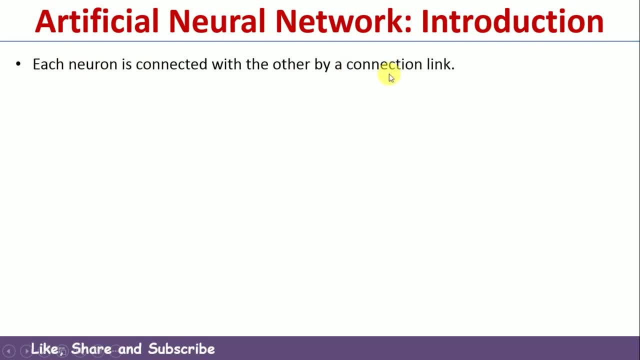 number of neurons. They are connected with one another. That connection is done with a link And each and every link is associated with a particular weight. Whenever we give a signal to a particular neuron, that input signal and the weight will be transferred to the next neuron. 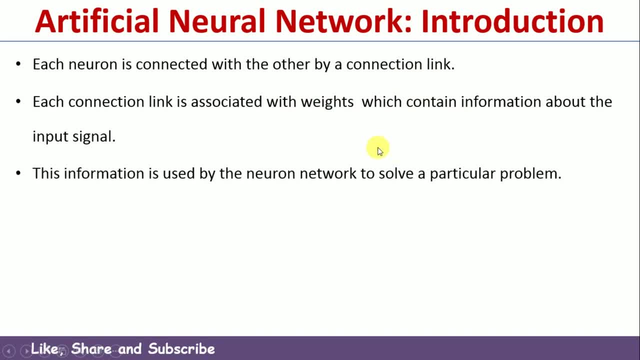 with the help of this particular link. in this case, This information, that is, the weight, whatever we have assigned to that particular link or whatever it is learned by that particular artificial neural network, is used to solve a particular problem. in this case, The artificial neural network is characterized by their ability to learn. 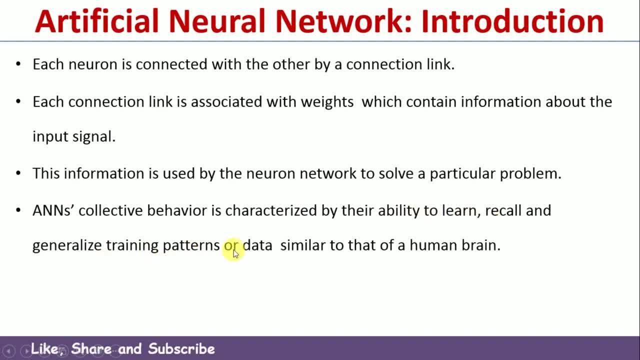 recall and generalize the training patterns or the data similar to the human brain. The way human brain works with the same node, the artificial neural network work like. they will learn and then they recall and generalize the training pattern over here. They have the capability to model the networks of original neurons as found in the brain. That's the reason these artificial 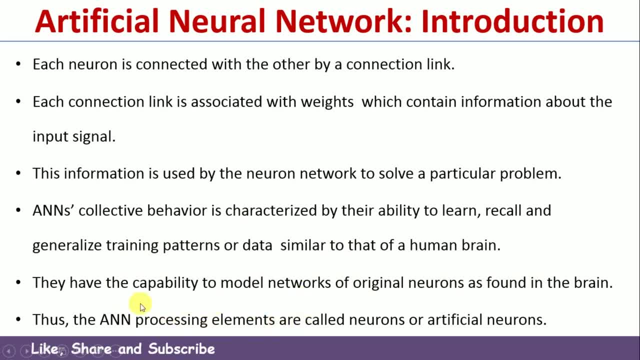 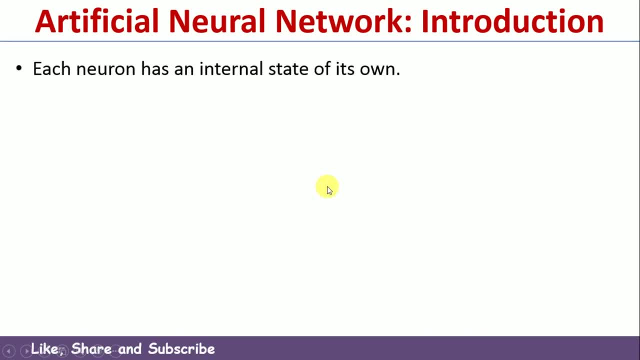 neural networks are called as the processing units of artificial neural networks are called as the neurons that are also called as the artificial neurons. in this case, Each neuron has an internal state of its own. As I said earlier, there will be multiple number of neurons in ANN. Each of them 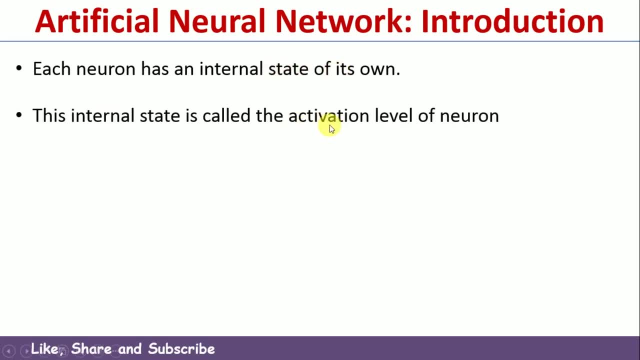 have their own internal state. That internal state is called as the activation level. That activation level is transmitted to other neurons with the help of the link. in this case. We will take a very simple example to understand the simple artificial neural network. In this artificial neural network we have two layers. The first one is called as the input layer. 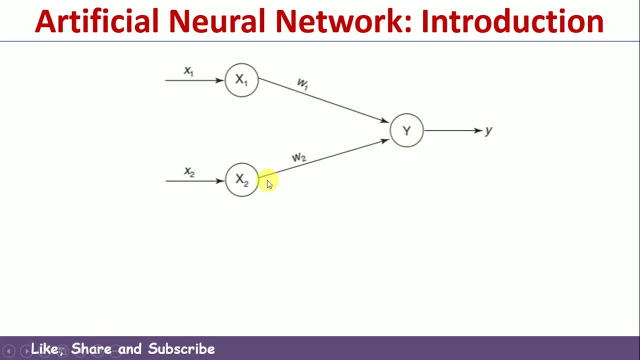 and there is another layer called as the output layer. These are the minimum two layers every artificial neural network has. In the input layer we have two neurons- that is denoted by x1 and x2, and y is the output neuron. in this case, That is, the output layer has one neuron and input. 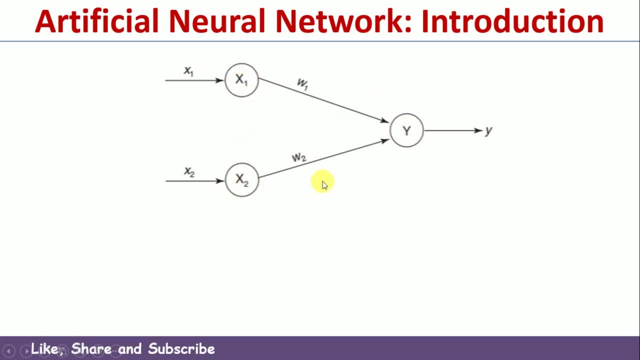 layer has two neurons. The total you we have three neurons in this particular neural network, And x1 and x2 are the inputs to this particular neuron and y is the output of this neuron. as I said earlier, each of these neurons are connected with the link. in this case, x1 and y is. 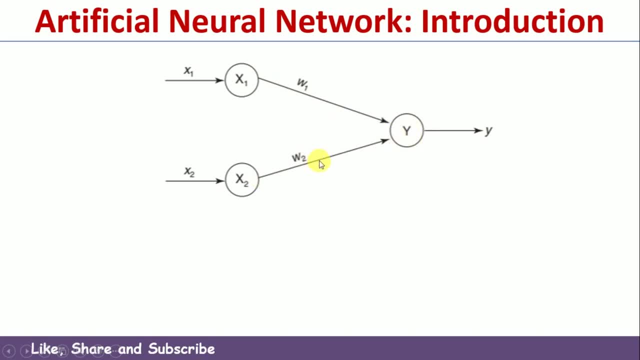 connected with this link. x2 and y is connected with this link and each and every link is associated with some width. Initially we assign some random width to each and every link and we perform some computation here. Finally, we will get to the hidden neuron region and we will able to get the actual shot cells in this gearовал. 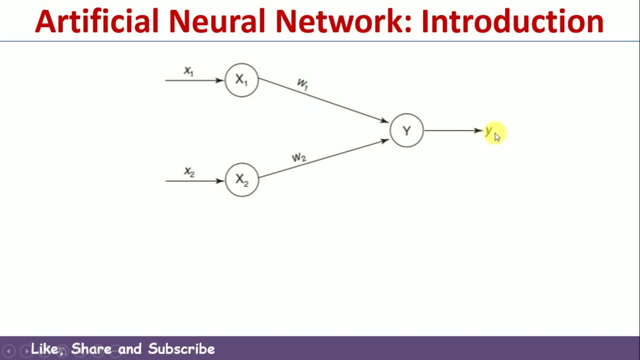 we will get this particular output. once we get this particular output or once the termination condition is satisfied, whatever the weight we have assigned to these two, w1 and w2, that is the final one. otherwise, if, if this termination condition is not satisfied, we have to go back. 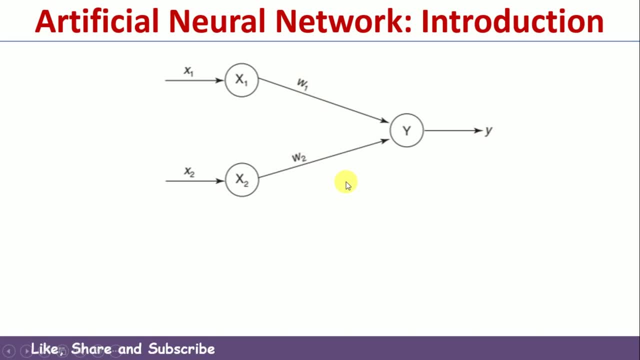 and modify these particular weights in this case. so to modify these particular weights we have some different algorithms like gradient descent, back propagation and so on. so we have to apply and update these particular weights in this case. now what kind of computation takes place in each and every neuron? is, for example, at this particular neuron y, the two kind of things takes place, or 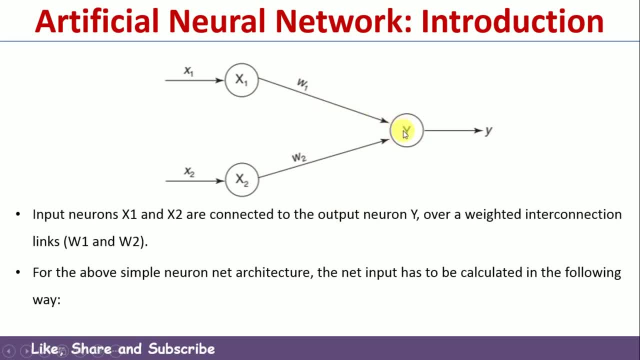 every neuron does these two things, that is, it performs something called as a summation, and then it performs something called as it will apply, something called as activation function, over here on the top of that particular summation. that is, summation is nothing but sum of product of. 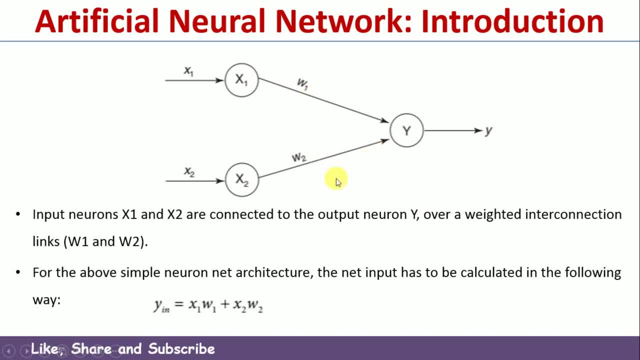 input and weight here. that is nothing. but you can say that y in is equivalent to x1, to w1 plus x2, w2 in this case. that is, x1 is input, w1 is the weight, x2 is the input, w2 is the weight in this case. now this is: